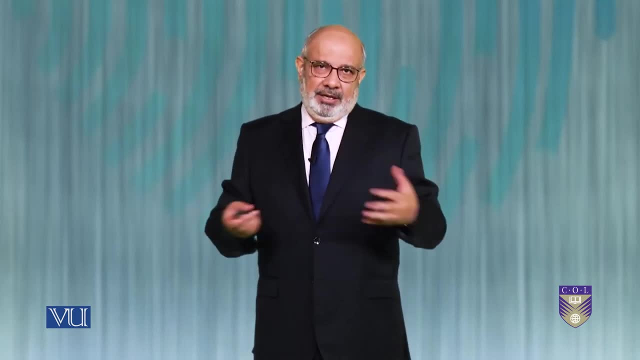 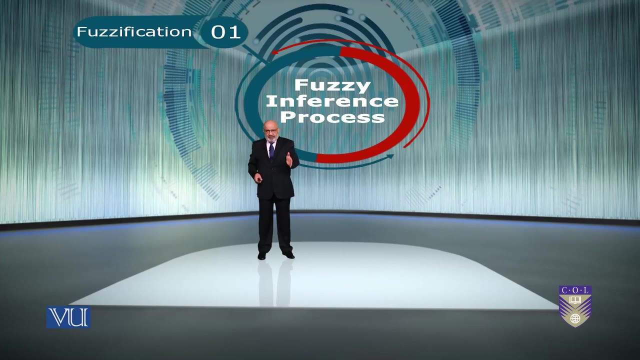 Input and output. In between is the fuzziness and the inference process. So what are the five steps? You start with the crisp input and you fuzzify that, fuzzify that, okay, We'll see what it is. And then we apply fuzzy operator on the premise or on the on the left. 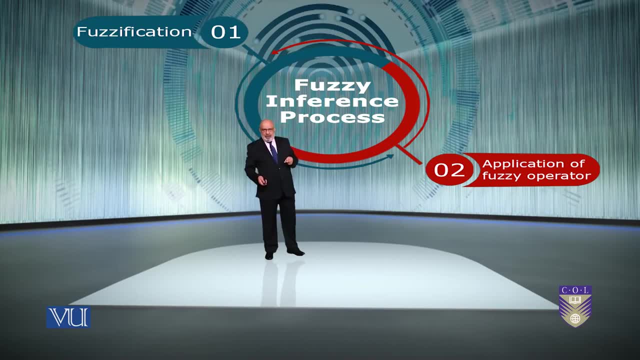 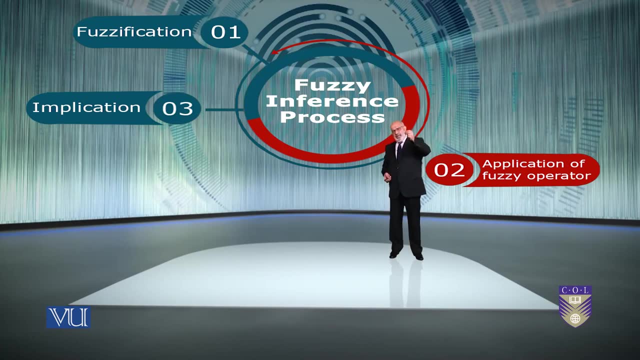 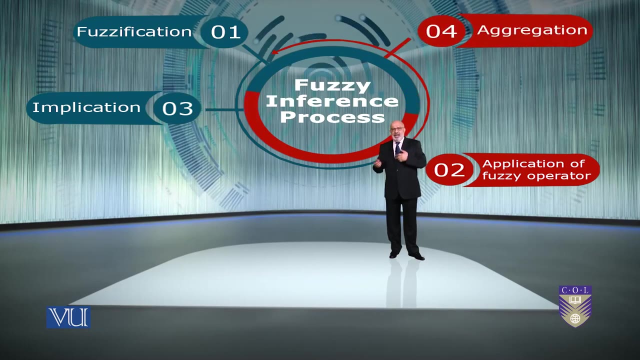 hand side of the rule. okay, Fuzzify, apply the fuzzy operator. okay, Then implication. implication is effectively the application of the rule. okay, So apply so from the antecedents to the consequent. then aggregation of consequences across the rule if you have multiple ones. 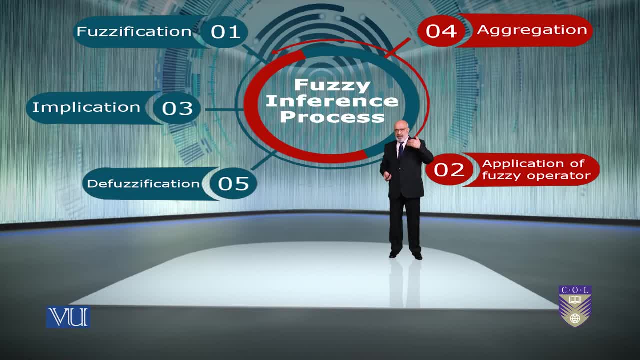 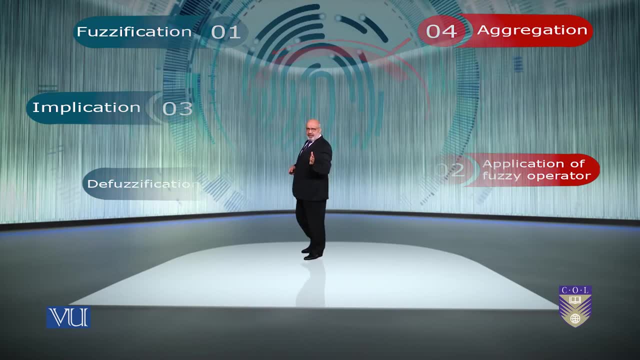 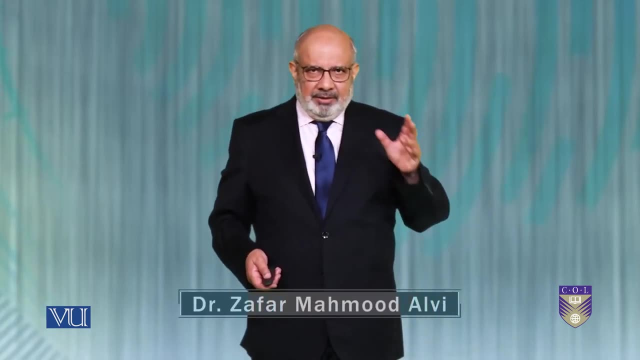 And then, of course, defuzzify So you come up with a crisp output. okay, So five steps We are. we are going to discuss subsequently a case study for a dinner- dinner for two people. okay, That's, a small case study will help you do that. Okay, So what? what exactly are we trying? 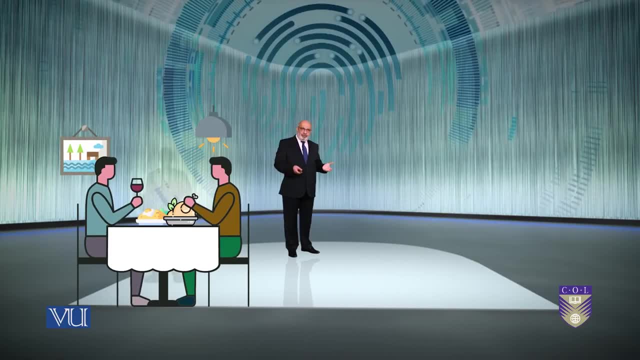 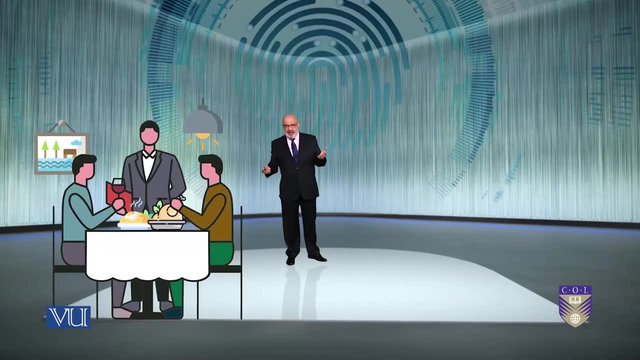 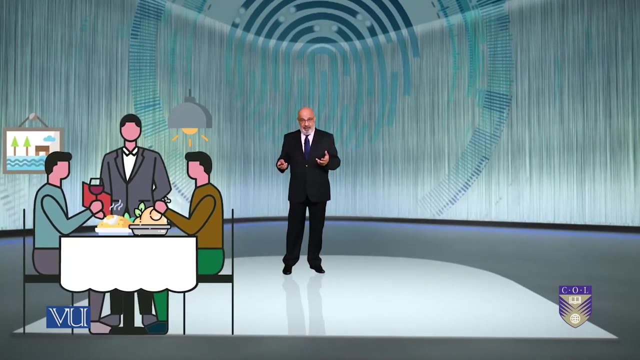 to do. We are saying, all right, the two, two people who want to go to a restaurant and then, depending upon what kind of food they get and what kind of service they get, okay, This fuzzy system will help them decide how much tip to give. okay, How do, how do? 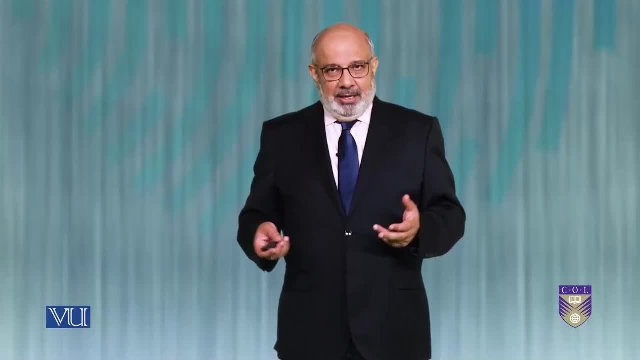 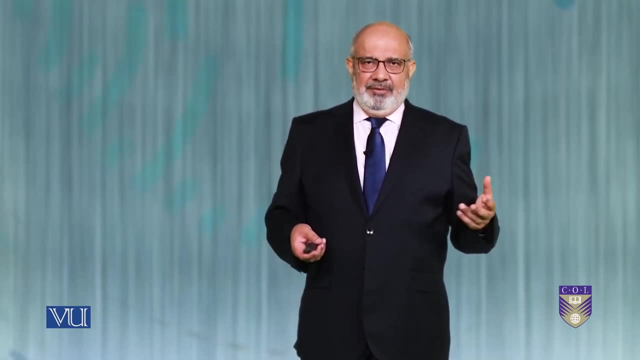 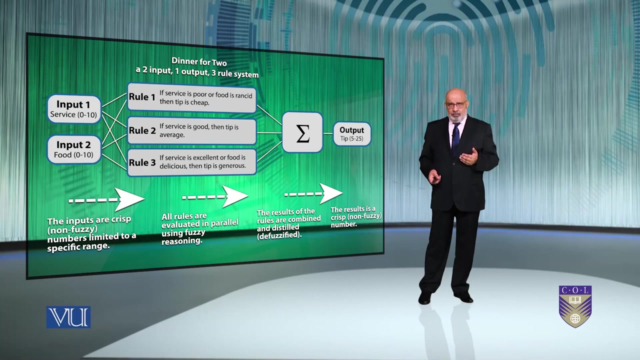 you tip off, tip the, the, the, the waiter. okay, It's a very standard thing And it can be a percentage of the total bill, Say, between five to 25% of the total bill. The system is based on three for the rules. Okay, We will discuss each one of them. rule: 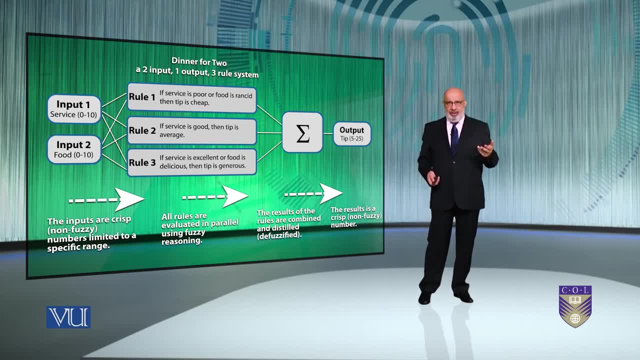 one, rule two and rule three, And then we will apply this, these, these three rules, and using the inference process. What's the first step? The first step is to create the error. That's the before-after패 rule, That's the following action. It's effective, The. 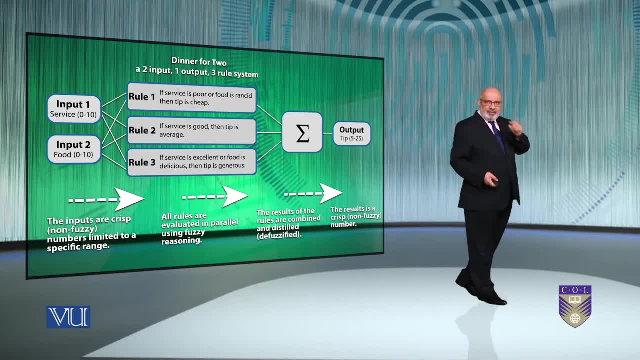 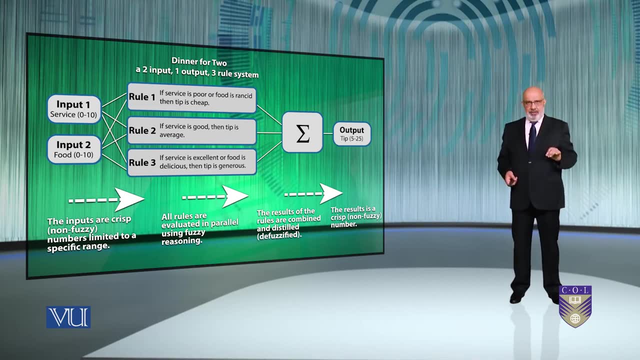 first step is this, And then the second step is to apply the error. The third step is to apply the error. That's First step is the fuzzification. So you take the crisp inputs and determine the degree to which they belong to each of the appropriate fuzzy sets via 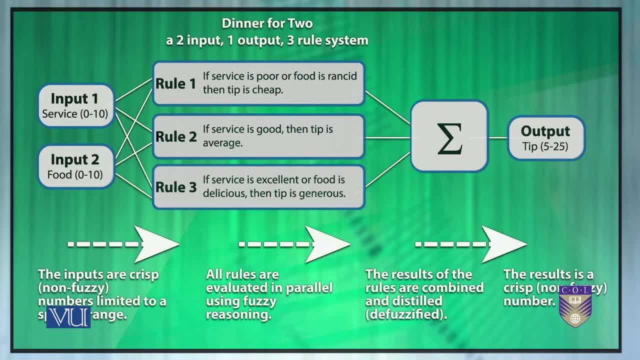 membership function. So in this case the numerical value of the crisp value. it can range between 0 and 10.. Okay, the service quality, you can say poor, mean mean 0 and 10 could be excellent. and the output, the fuzzy degree of membership, using the linguistic set of variable, will be in the range of 0 and 1.. So 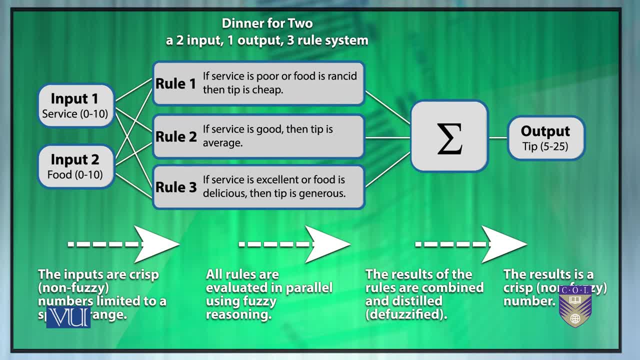 fuzzification of the input is either through a lookup table or a fuzzification function I mentioned previously, Of course, built using three rules, and so you fuzzify the inputs. Once you are fuzzified, your next step is how to actually apply those rules. the implication, So left-hand side of the 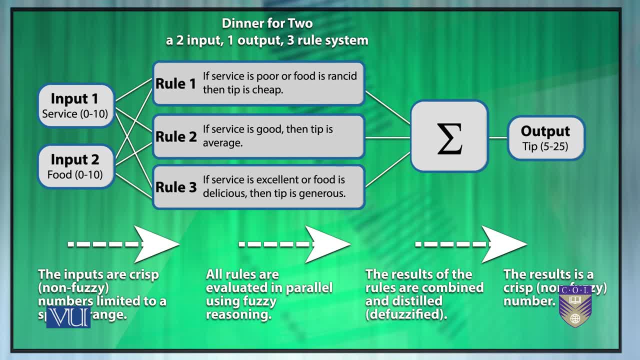 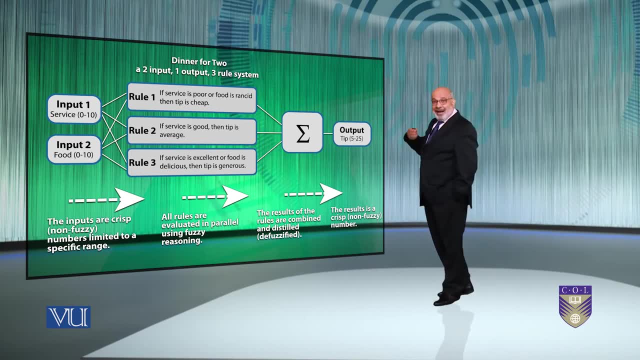 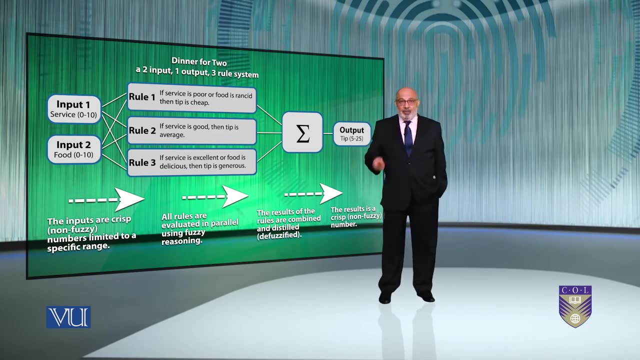 rule, which ones, and then the implication of each rule. So, for instance, what is the extent to which the food is delicious, and the figure will demonstrate how well the food of our hypothetical restaurant qualifies on a scale of 1 to 10. 0 to 10.. Okay, and the linguistic variable here is: 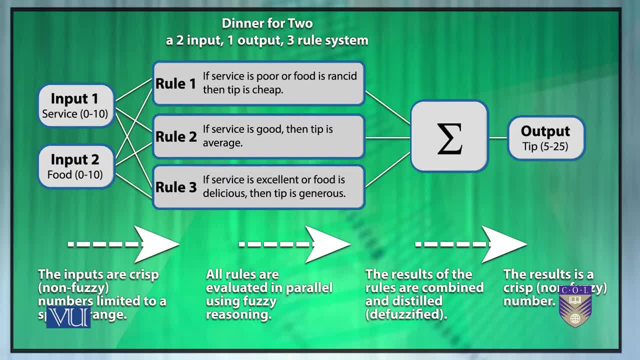 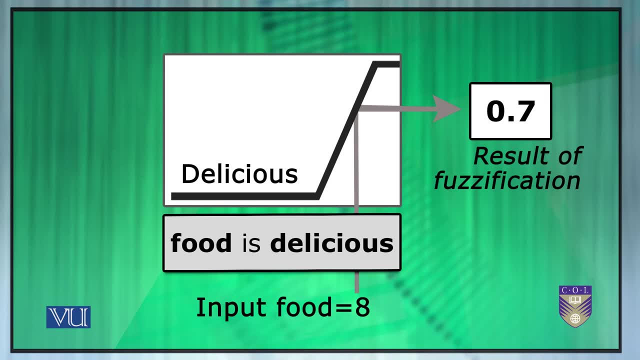 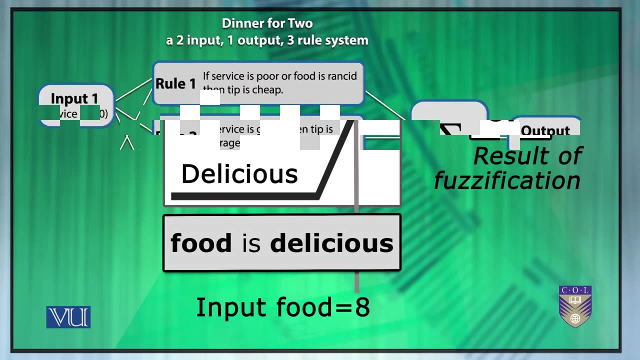 the word delicious the food quality. So the diners have rated the food as as an 8. well, and given the graphical definition of the delicious, that corresponds to value of 0.6.. 0.7 of the delicious membership function. Now we apply the fuzzy operator once the 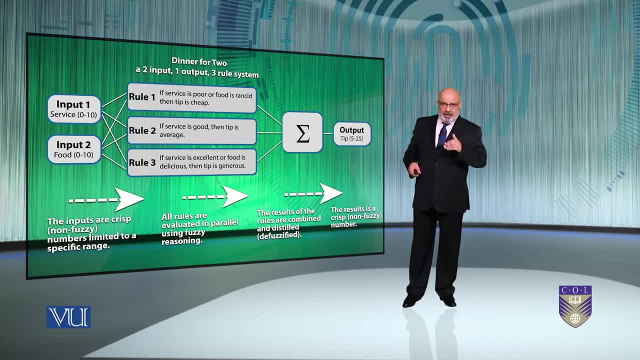 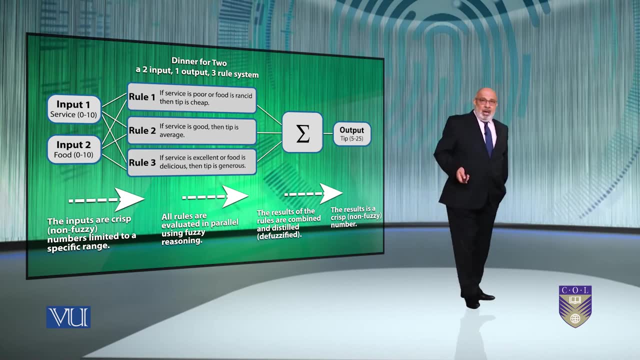 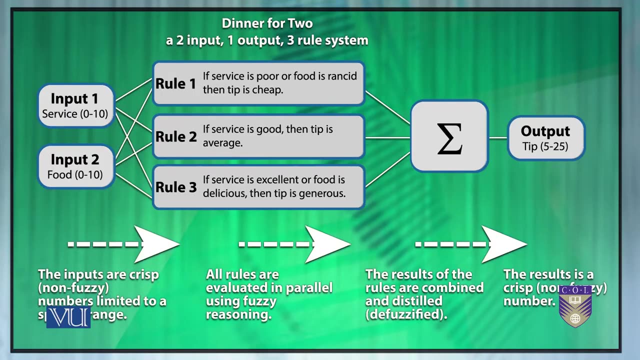 inputs have been fuzzified and we know the degree to which each part of the left-hand side or the antecedent has been satisfied. for each rule, we apply the fuzzy operator. Now, once the fuzzy operator is applied, we then actually aggregate them. okay, So each rule is applied if there are more. 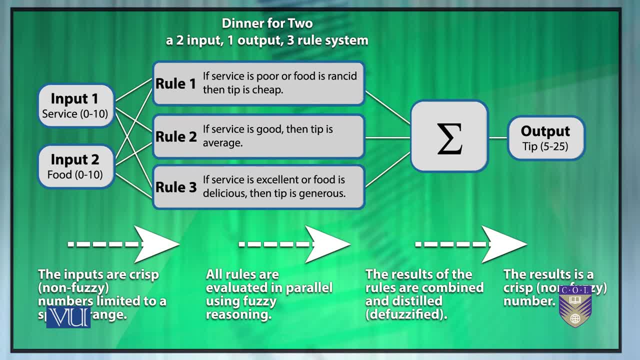 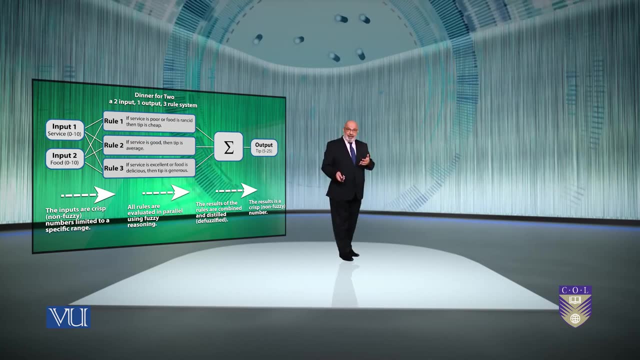 than one left-hand side, remember, and or all kind of thing. So and would take the minimum and the odd would take the maximum if there are more than one. So fuzzification, followed by the implication, So fuzzy sets, and then rules applied, and then they aggregate it. So, once again, what are those five steps?